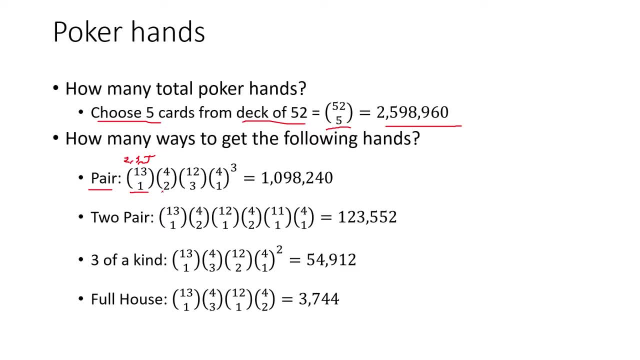 pair And then we choose a suit for our pair. And then we choose a suit for our pair And keep in mind that each card in the pair is going to have a different suit. So we choose two of those from four, And by suit I mean like diamonds, spades, clubs, etc. Or hearts. 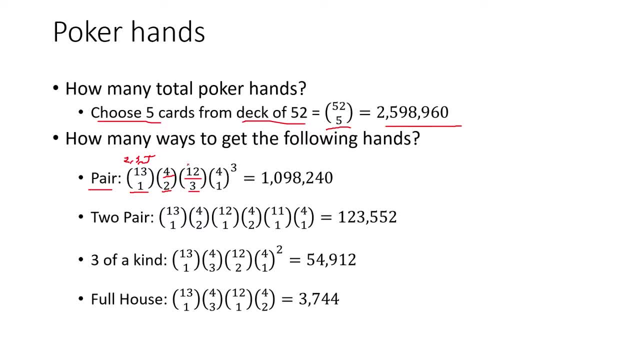 Next we choose the remaining cards, So that'll be 12- choose 3.. And then we're going to choose a suit for each one of those, So there's four possible options to choose from, and then we have one suit per card. And then we repeat that three times and that'll get us around. 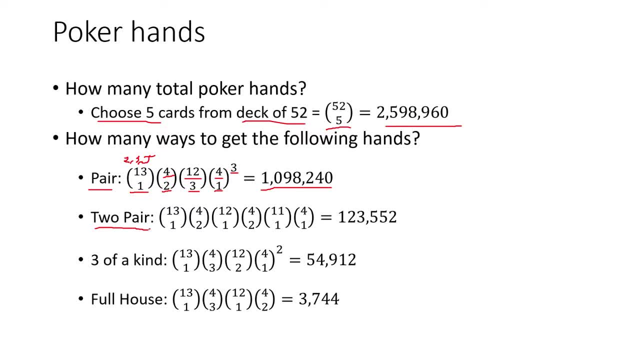 a million. Likewise, we do the same computation with the two pair. We first choose the rank of our first pair, And then we choose suits for each one of those cards, And then we choose the rank of our second pair, And then we choose a suit for each one of those cards, And then 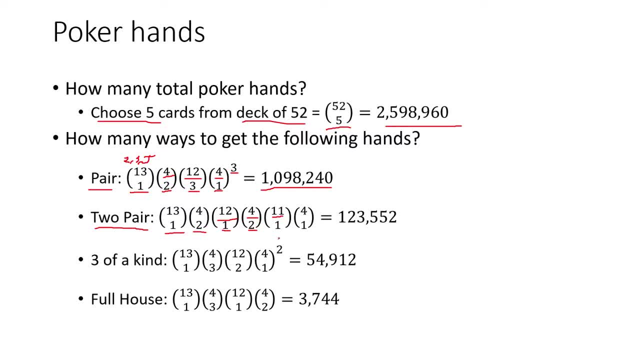 we choose one more rank for the remaining card out of 11.. And keep in mind that this number decreases each time because we've already used a rank in the previous pair And then we choose a rank here And that gets us around 123,000.. So next is going to be a three of 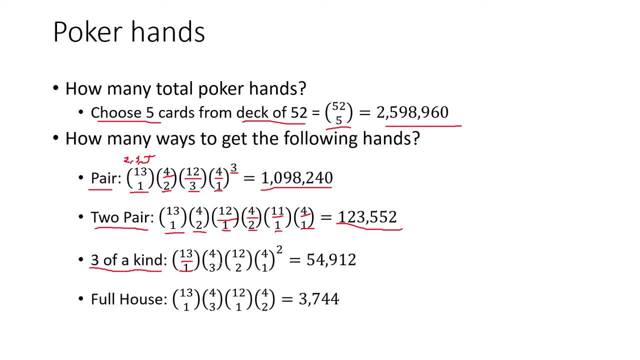 a kind: We first choose a rank for our three cards, And then we choose a suit for each one of those, And then we can choose a rank for the remaining two cards- Notice that they have to be different- And then we choose a suit for each one of those, Because there's 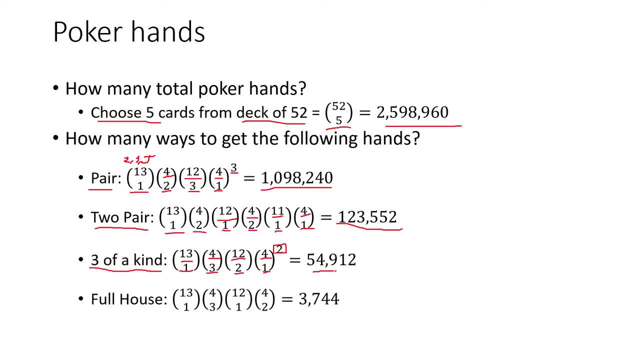 two cards. we square this quantity here And that gets us around 55,000.. So next is going to be a three of a kind, And then we're going to choose suits for our three of a kind, And then we're going to choose a rank for our pair. Notice that one rank has already been. 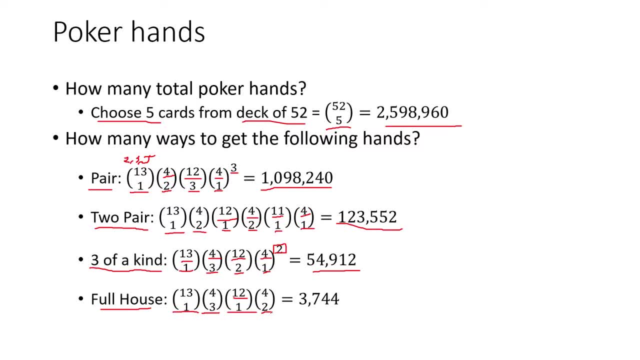 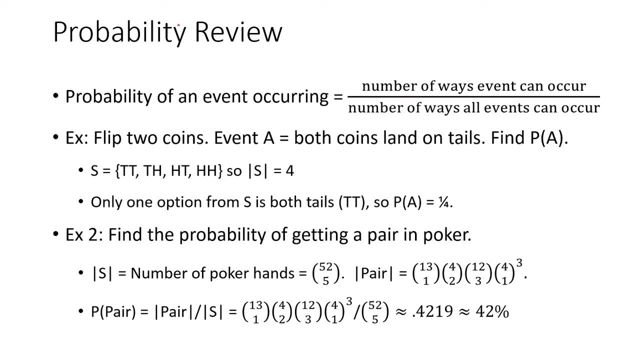 used And then we're going to choose suits for each one of those cards in our pair And that will give us around 3,700.. This is just a quick review of probability. The probability of an event occurring is going to be the number of ways an event can occur versus the number of ways all events can occur. 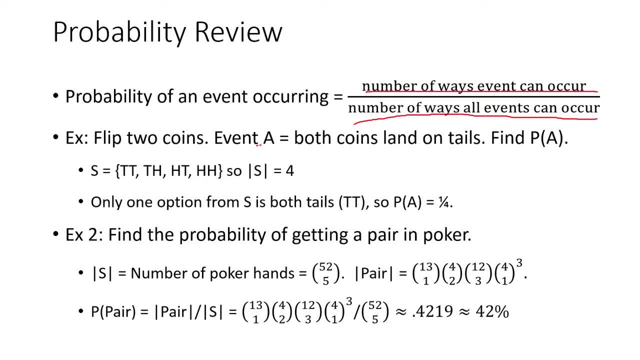 So a simple example would be flipping two coins. Let A represent the event that both coins land on tails. We're going to go ahead and compute the probability of that, So we're going to first list off all the possible ways coin flips can happen. So we have tails, tails. 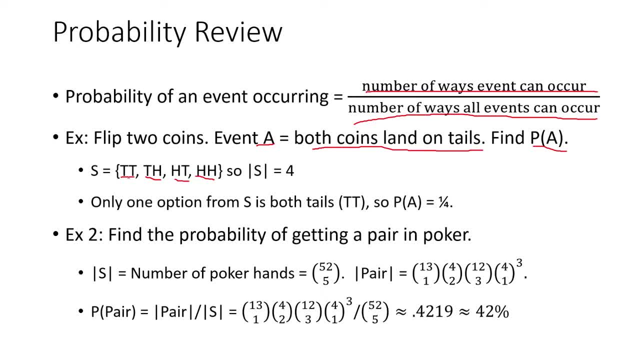 Tails, heads, Heads, tails And heads, heads, And we're going to put all of these in our set S, which is going to represent our sample space, And if we compute the cardinality of S, we can see that it's simply four. 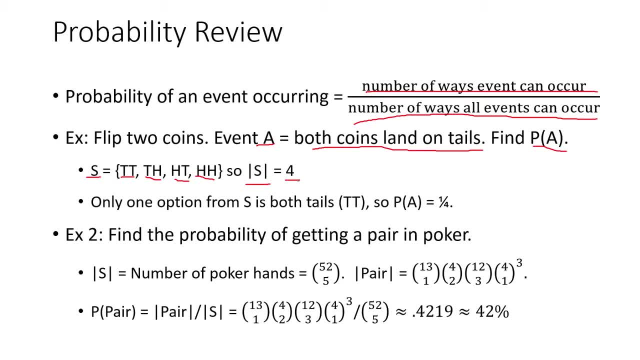 So that's the number of ways all the events can occur. So notice that only one option from the sample space is both tails, That's the tail tails I just boxed off there. So that means the probability of both coins landing on tails is going to be one over four. 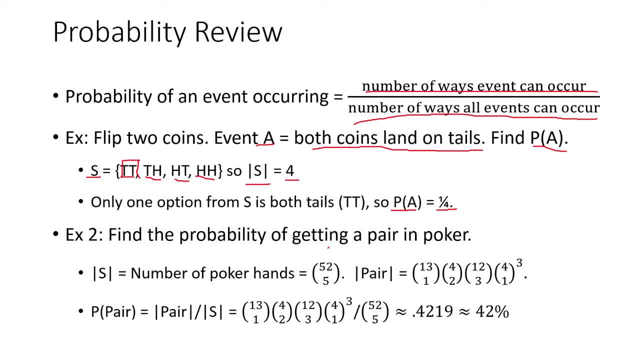 So another example: using the values we computed previously, we can find the probability of getting a pair in poker. So we're going to let the cardinality of tails be one over four. So we're going to let the of S be the number of poker hands possible, and we computed that to be 52, choose 5.. Next, 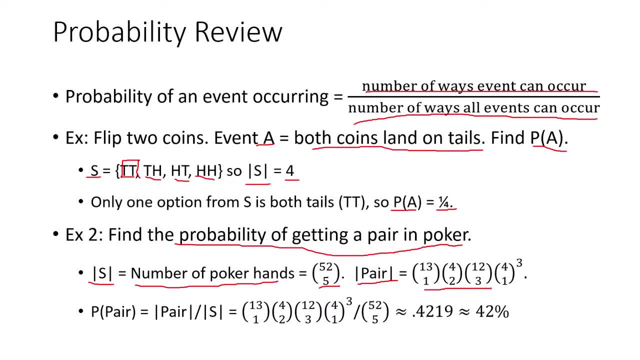 we're going to compute the number of ways we can get a pair and that's this quantity right here. So the probability of getting a pair is going to be the number of ways we can get a pair over the number of possible poker hands. and once we crunch the numbers, 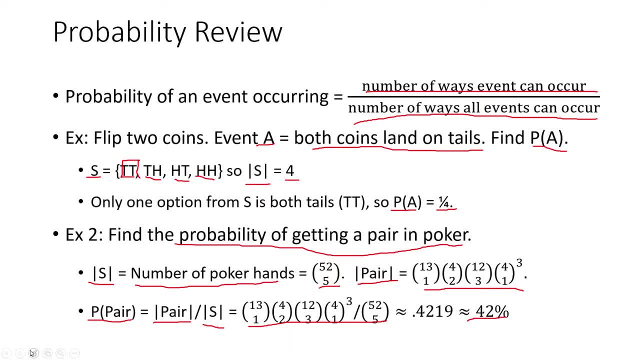 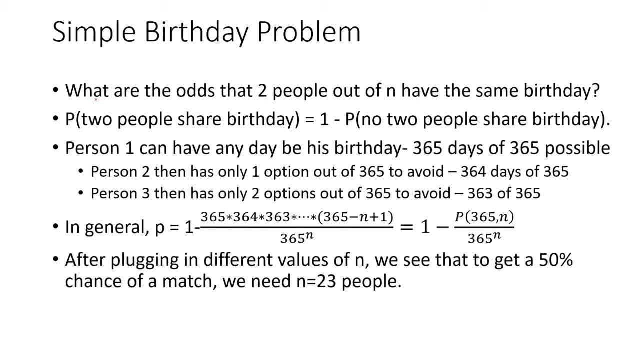 we'll see that it comes out to around 42%. So another example is going to be the birthday problem, and that's simply computing. what are the odds that two people out of N have the same birthday? Now notice that the probability of two people sharing the same birthday is. 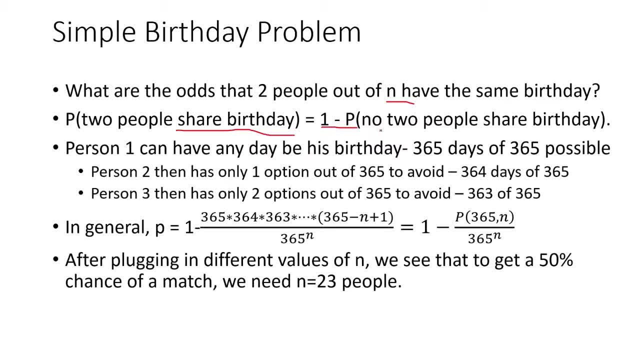 the complement of the probability that no two people share the same birthday. right, because those are opposite events. So one way we can compute this, this quantity on the right here, is we can first assign a day for person 1, and they could have a day for. 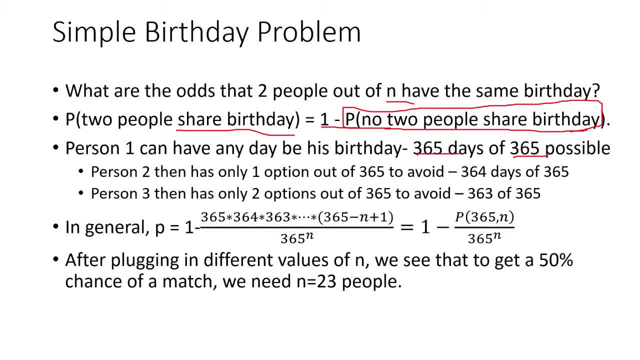 3, and they could have any of the days out of the year, 365 out of 365 possible. Person 2, on the other hand, has one option to avoid. that's the day that person 1 chose, So that leaves him with 364 days to choose from. Then person 3 has two options to avoid, right. 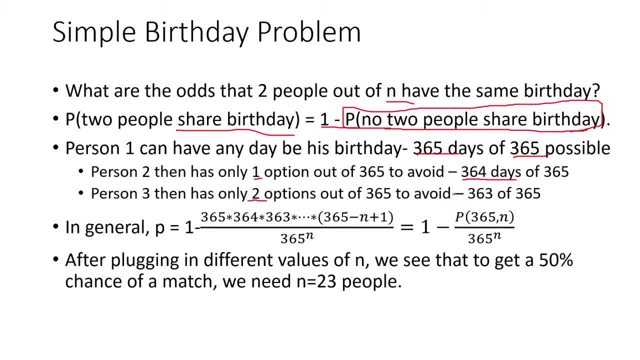 whatever person 1 has and whatever person 2 has. so that leaves them with 363.. And we can repeat this several times and we notice that we'll get a pattern as seen in the new numerator. here We'll have 365 times 364, all the way down to 365 minus N plus 1.. That's. 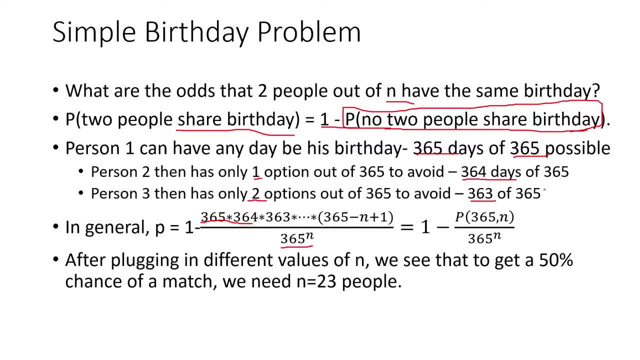 all going to be divided by 365 to the N power, and that's just from the right hand side here, And we'll simply notice that this numerator here can be expressed as a permutation. So we can simplify this down into 1 minus the permutation of 365 and N divided by 365. 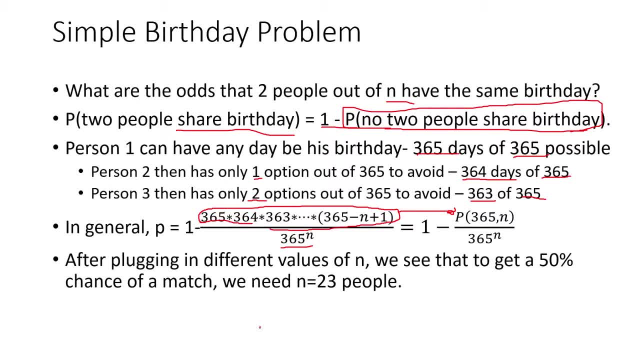 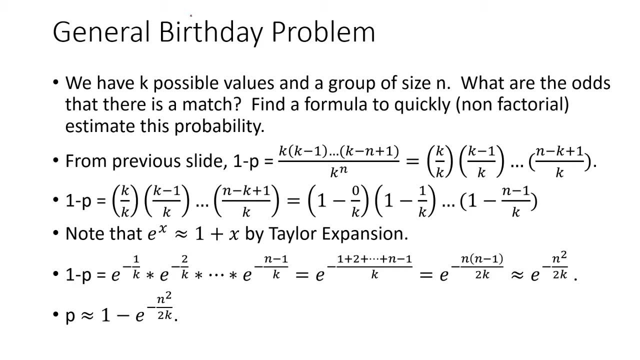 to the N, And after we plug in different values of N to this formula, we can see that there's a 50% chance of a match with 23 people, which is a little bit unintuitive. So next we're going to move on to the general birthday problem. Now, instead of 365, we're going to 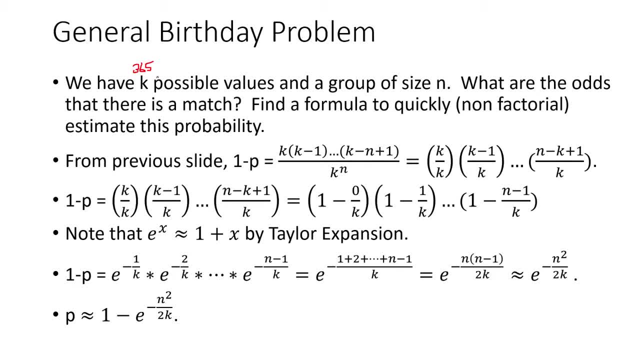 have k just be an arbitrary variable. So before this was days, But now we're just going to make it k possible values and we're going to take it out of a group of size N- Remember this was N people from the previous example. So now what are? 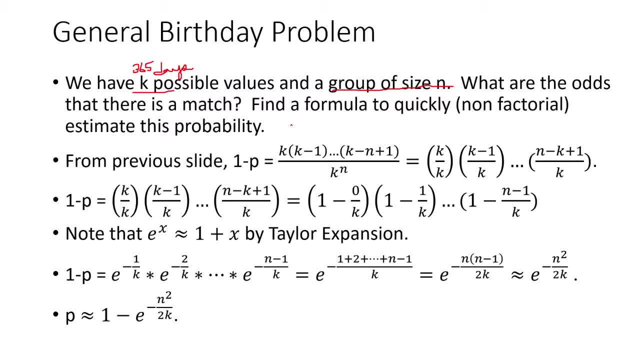 the odds that there's a match And we're going to quickly find a formula to quickly estimate this probability, because permutations and what not, and factorials can blow up very quickly. The numbers can get very large. Sometimes it'll overflow the calculator or the computer. 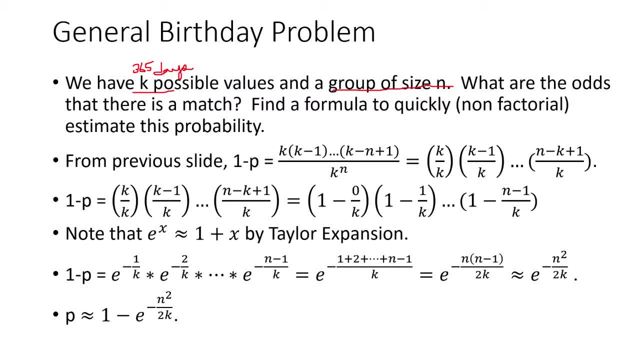 So we need to find a quick way to estimate that. So we're going to go ahead and use what we know from the previous slides, that our probability here can be represented as k over k times k minus 1 over k. Remember this was like 365. 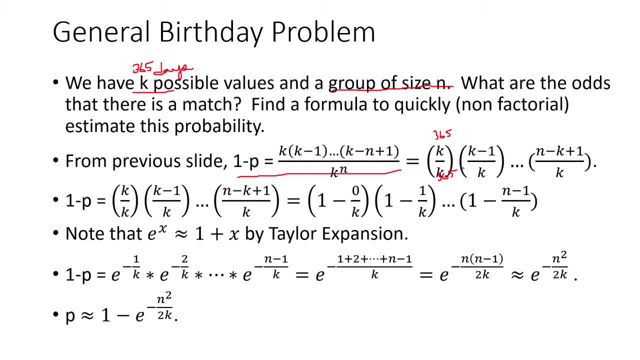 over 365, 364 out of 365,, et cetera, And we'll notice that the probability here is going to be the number of times that it's going to be 0, the number of times it's going to be 1,. 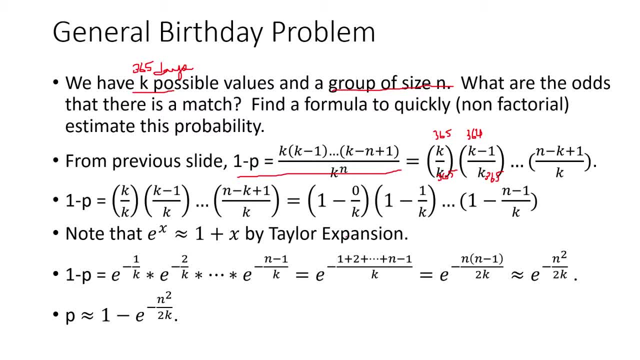 and then the number of times that it's going to be 0, and then the number of times that it's going to be 0. We're going to take our probability here And we'll notice that that can be rewritten if we simply divide through the k to this: 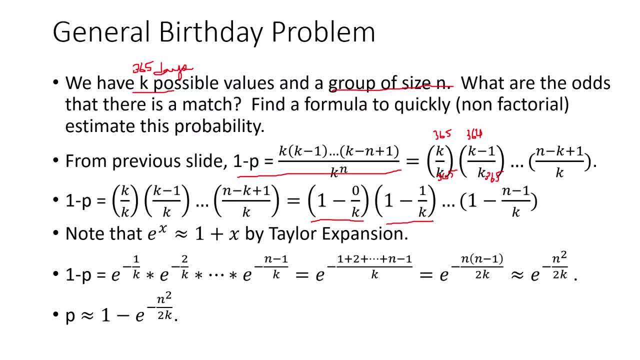 right here We'll have 1 minus 0 over k times 1 minus 1 over k times 1 minus M minus 1 over k, And we can recall that e to the x is approximately 1 plus x by using a Taylor.